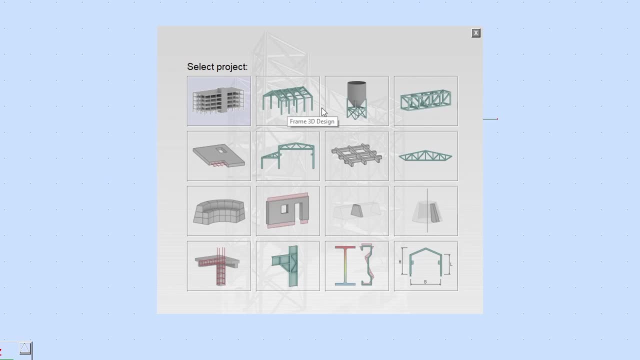 What is cool about the Robot is that it gives you the option to select beforehand the type of project you will be designing, and it will optimize the user interface for that area of focus. Robot supports many design codes like American, Australian, Eurocode. 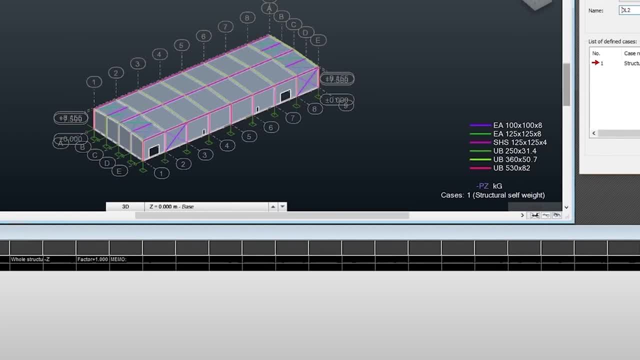 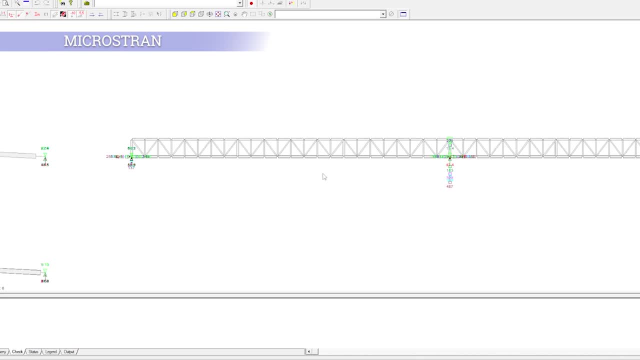 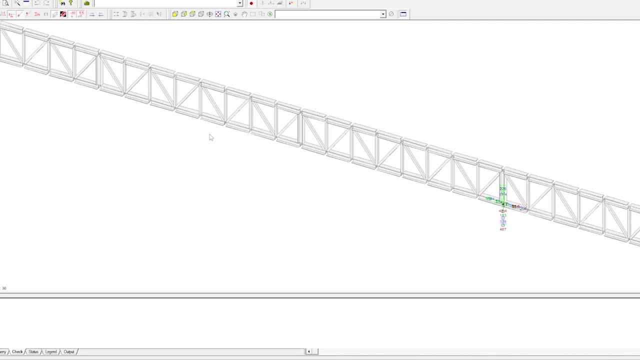 and many more. I use Robot to analyze and design the same type of structures as for Space Gas. Third on the list is MicroStrand from Bentley, which is the same company of RAM Concept MicroStrand. MicroStrand is also a general-purpose structural analysis package which offers a built-in 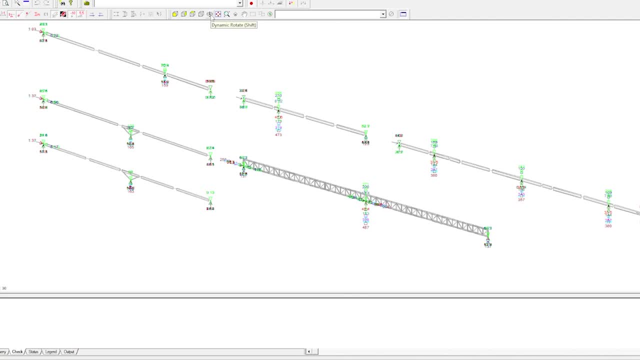 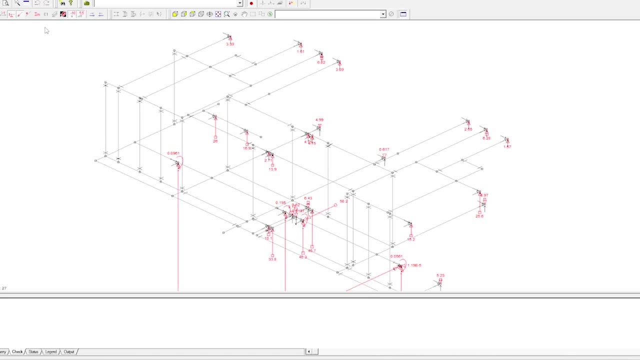 steel member and connection design. We use this software in the office that I'm working because it's part of Bentley's package. It does the job when it comes to structural analysis, but I'm not gonna lie, the graphical interface leaves a lot to be desired and it's not my favorite one. 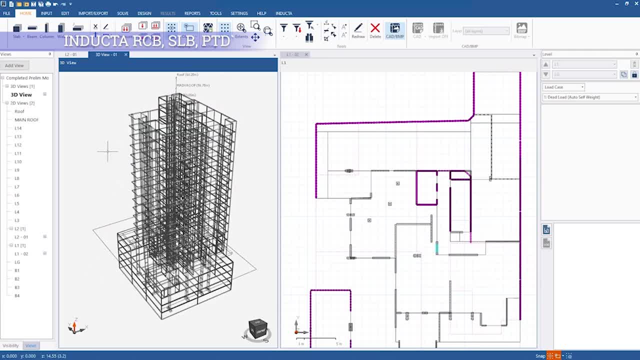 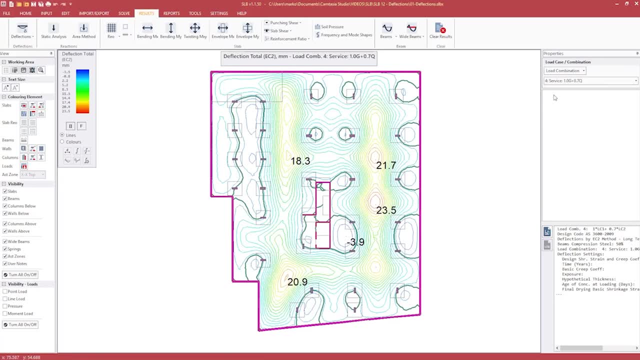 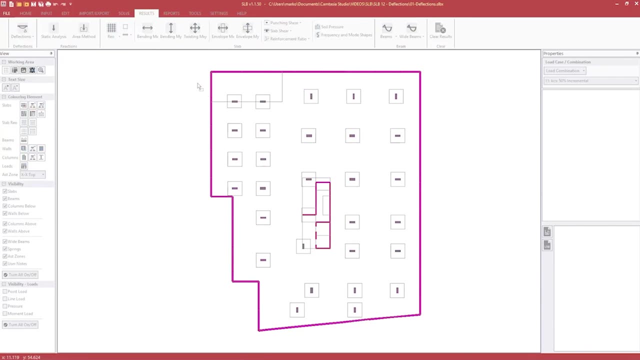 The fourth one on my list is the Inductor package. They are finite-element software for the analysis and design of reinforced and post-tension concrete structures. I usually model the whole building in RCB to assess vertical and lateral loads and then export the slabs to SLB or PTD for the design. 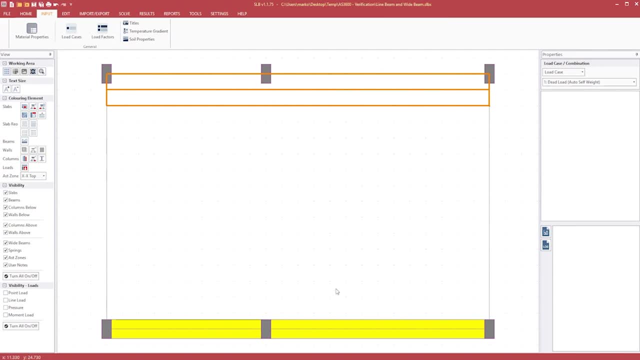 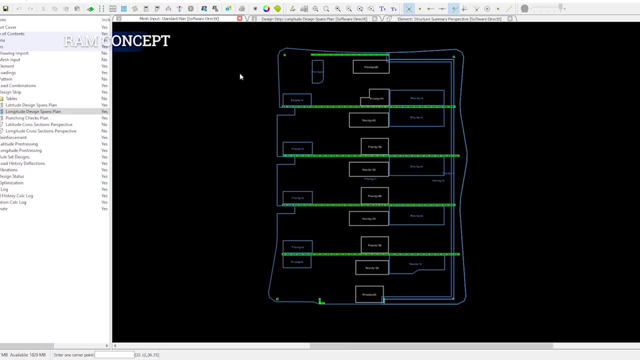 I find the user interface quite intuitive and the software is very easy to learn. I would definitely recommend this software if your focus is on concrete buildings in Australia. The fifth on the list is RemConcept from Bentley. It is also a powerful finite-element software. 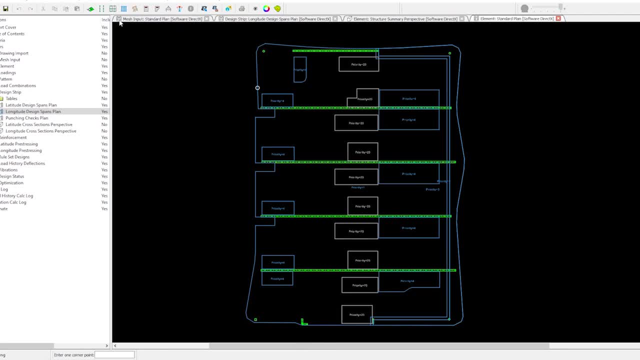 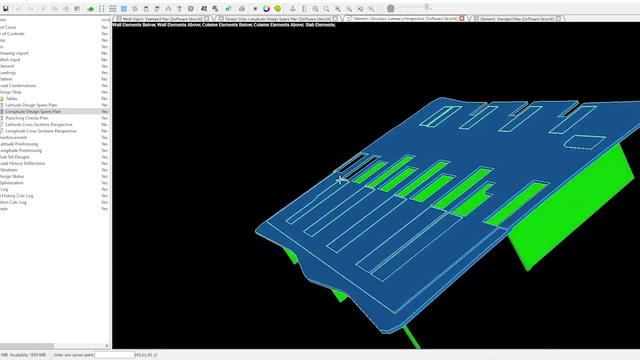 RemConcept is a finite-element analysis tool for the design of reinforced and post-tension concrete slabs. Rem has this process of defining design strips, which is essential that you understand before starting using the program. I've been using it recently at work and it's quite fun to design with this tool and I 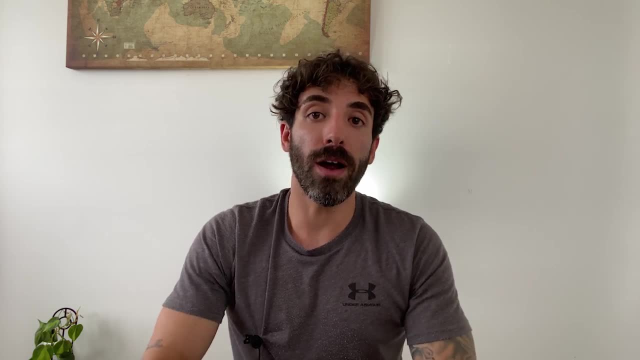 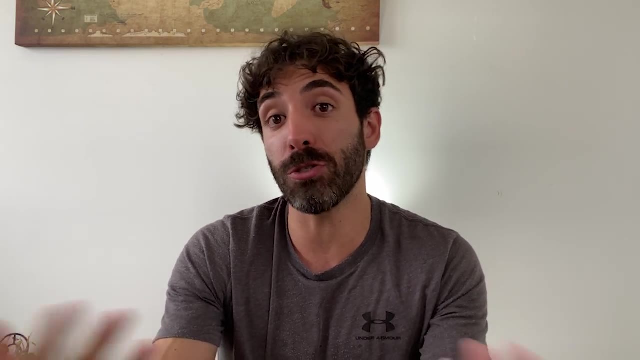 also recommend it for concrete buildings. The next two software on my list are three very specific and straightforward to use. I decided to add them here because I use them a lot at work. Unfortunately, they are applicable only to all. I'm not going to talk about them in this video. 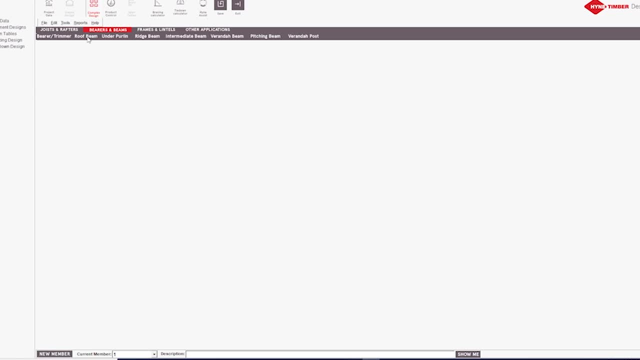 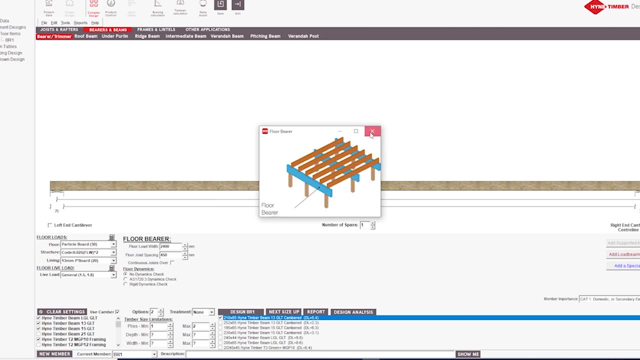 I'm going to talk about them in this video. I'm going to talk about them in this video. I'm going to talk about them in this video. The first one is Hein, which is a structural timber design software. The program includes engineering properties of the most popular Australian engineered.